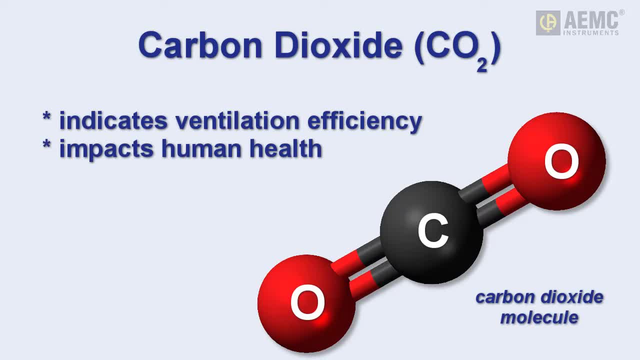 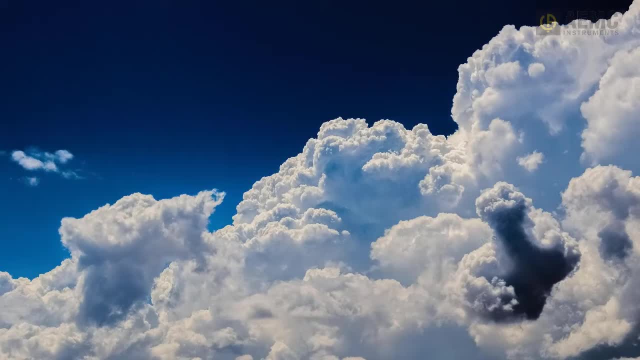 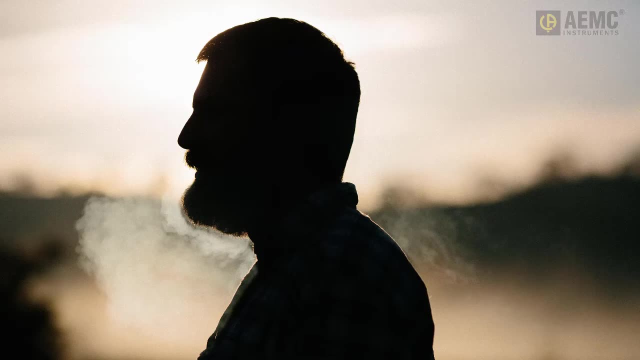 both as an indicator of the efficacy of a building's ventilation system and for the adverse impact carbon dioxide itself can have on human health. Carbon dioxide is a colorless, odorless gas that is a natural component of the atmosphere. It is also a byproduct of human breathing. 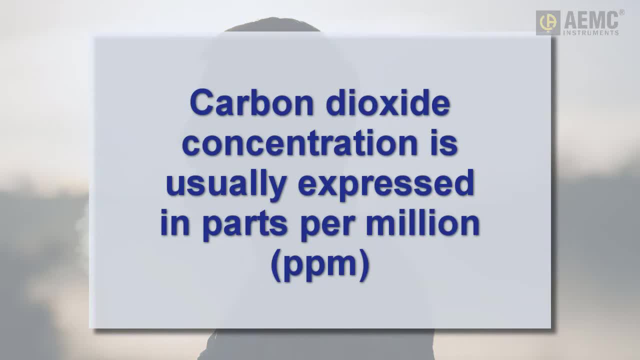 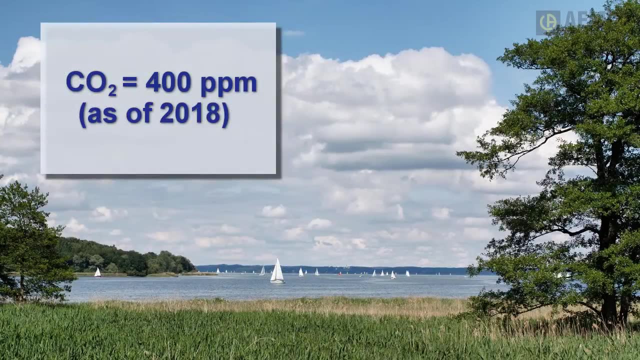 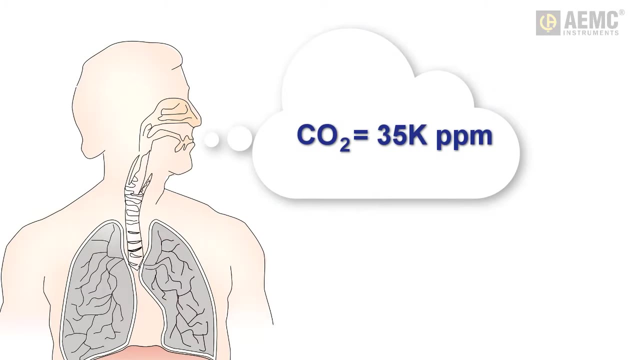 The amount of carbon dioxide in a given air sample is typically expressed in terms of parts per million. The ambient air in most outdoor locations around the world contains approximately 400 parts per million of carbon dioxide, While each exhaled breath of an average adult contains 35,000 or more parts per million. 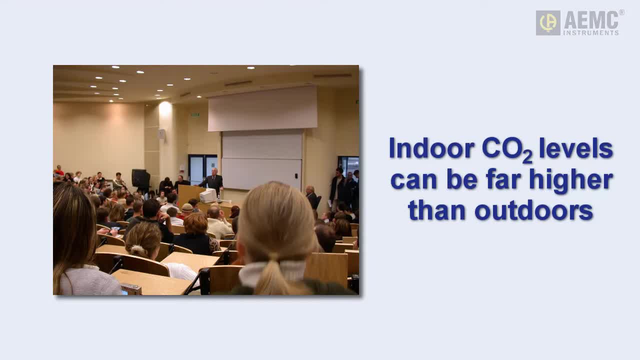 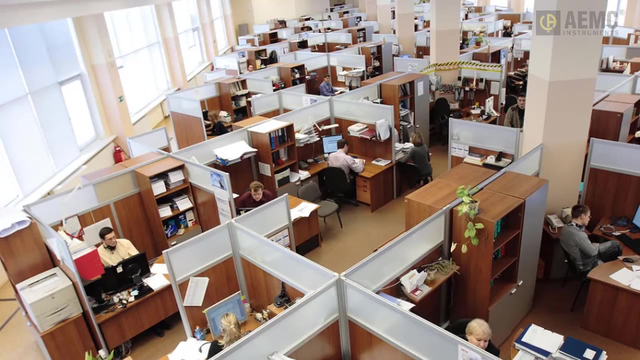 As a result, indoor levels can be considerably higher than outdoor, especially in facilities such as workplaces and schools, where large numbers of people spend the day in close proximity, Without adequate ventilation to dilute and remove the carbon dioxide being continuously generated by building occupants. 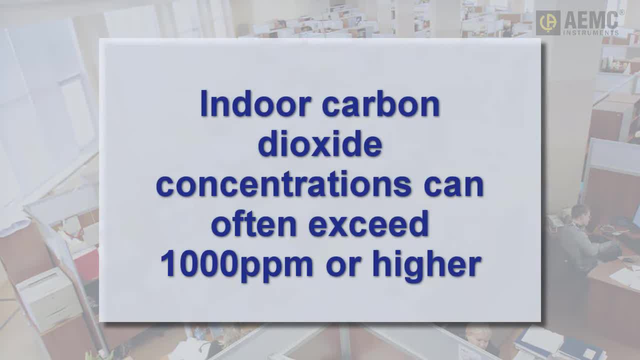 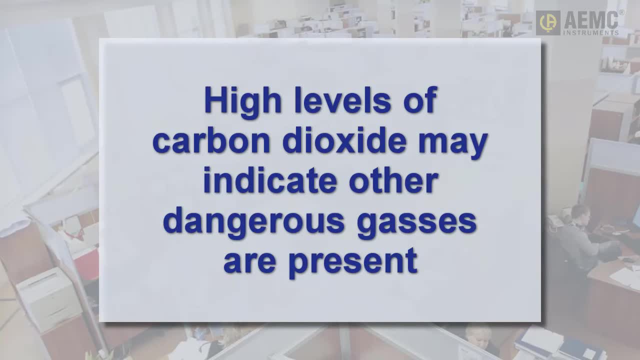 it can accumulate well beyond the 1,000 parts per million level and in some cases far higher. The amount found within an indoor environment is often used as a marker for whether other gases' pollutants are likely to become a nuisance or hazard. 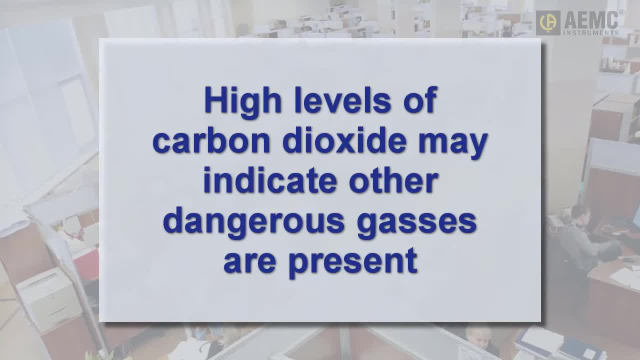 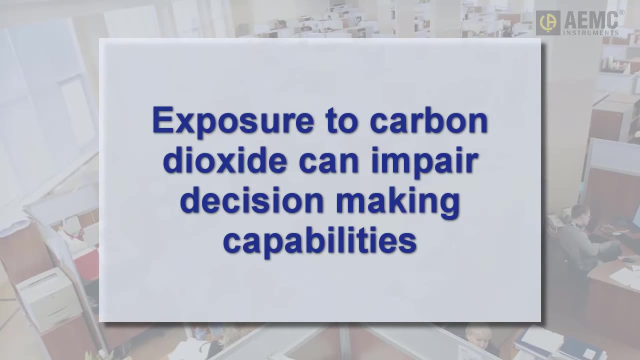 And although carbon dioxide is not usually considered toxic, recent research is raising concerns about the detrimental effects heightened levels of this gas may have on people. For example, a US government survey found that moderately high indoor concentrations of carbon dioxide can significantly impair a person's decision-making capabilities. 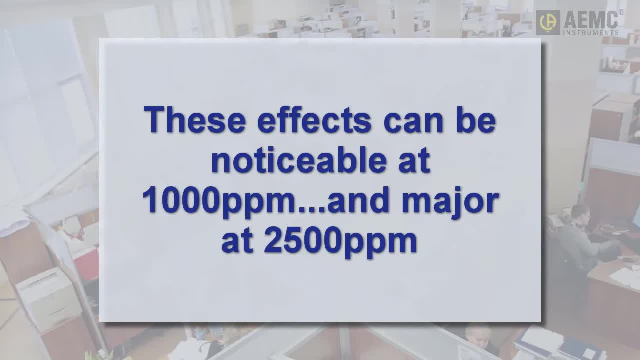 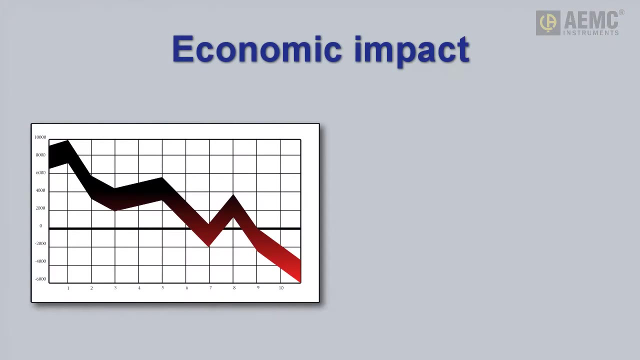 Test subjects showed significant reductions in performance at carbon dioxide levels- around 1,000 parts per million- and large reductions at 2,500 parts per million. This shows that even moderately elevated levels of indoor carbon dioxide can adversely affect us. Indoor air quality can also have an economic factor. 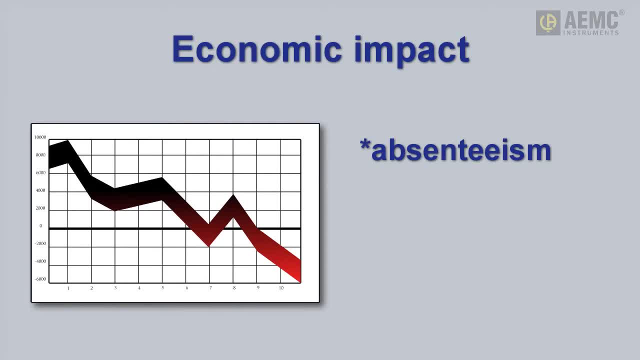 Absenteeism, discomfort and lowered productivity can directly impact employee performance, And elevated levels of pollutants may indicate that your ventilation system is running inefficiently and wasting energy. Fortunately, as environmental sensors become widely available, indoor air quality is no longer an academic pursuit. 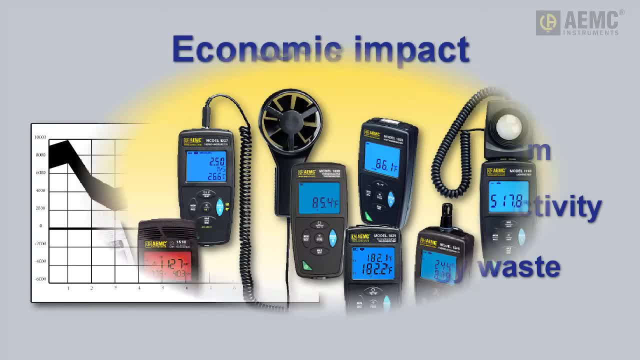 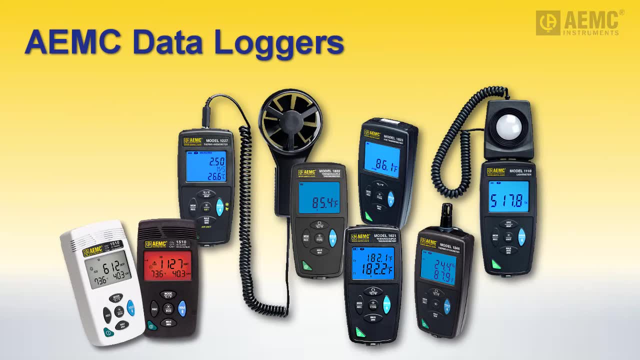 but something building managers and others can track and control. For example, AEMC offers a variety of data loggers that can help you monitor indoor environments for occupant health and comfort. One such instrument is the Air Quality Logger Model 1510,. 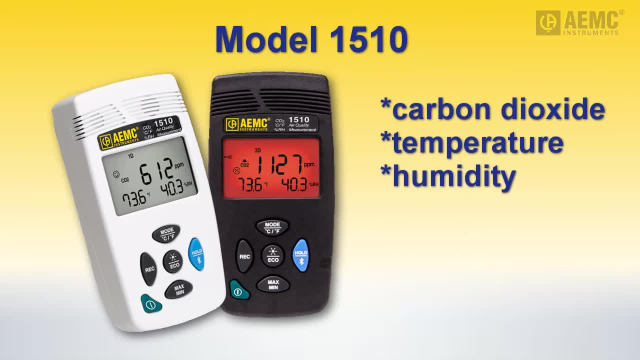 which monitors carbon dioxide, temperature and humidity in the local air. This compact, easy-to-use instrument provides quick and accurate readings and can store up to one million separate measurements. The Model 1510 features adjustable alarm settings for indicating when measurements fall outside a specified range. 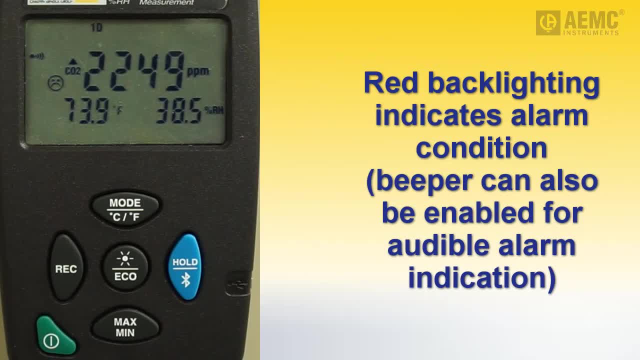 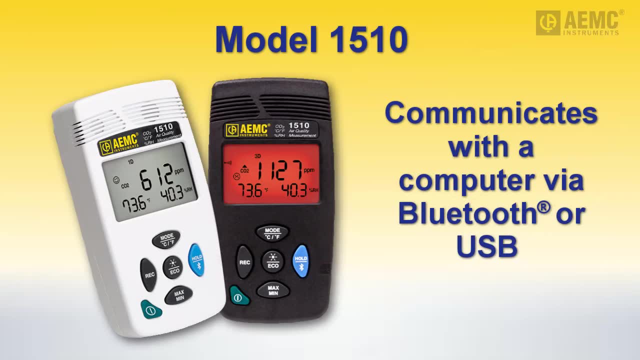 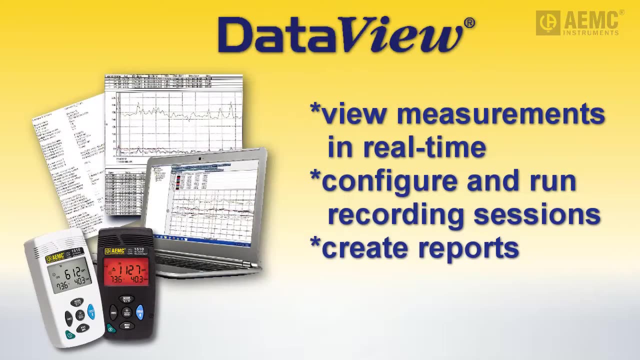 The display blinks with red backlighting when any of the measured parameters exceeds user-selected thresholds. The instrument includes USB and Bluetooth communication for downloading recorded data to a computer. The Model 1510 is also supported by AEMC's DataView data analysis software for viewing real-time data. 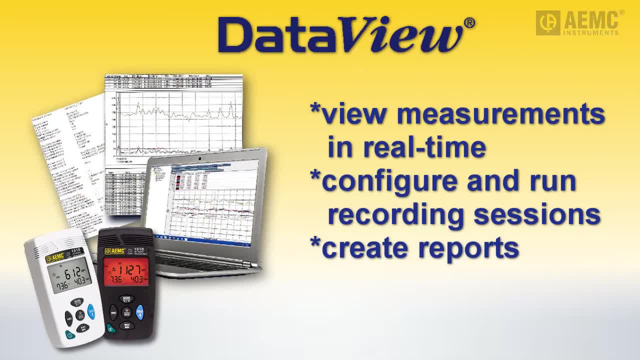 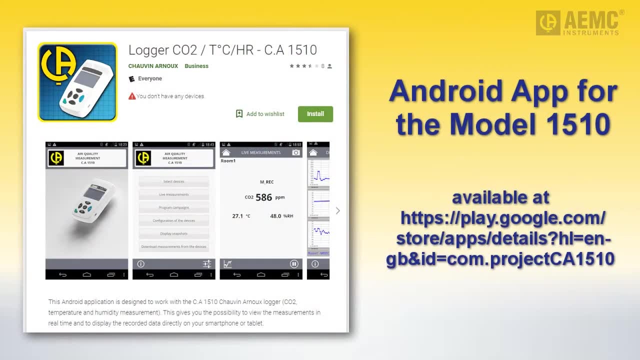 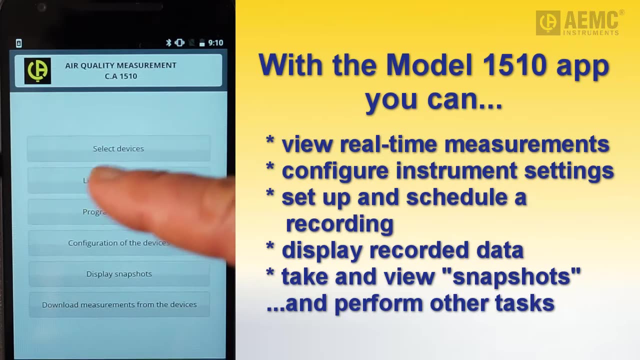 configuring and running recording sessions and creating reports. These reports can then be saved and reviewed for identifying and analyzing long-term trends. The instrument is also accessible via a free Android app. This allows you to view measurements in real-time. display recorded data. configure the instrument. 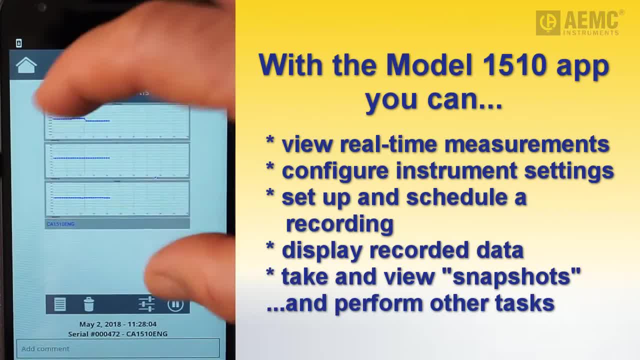 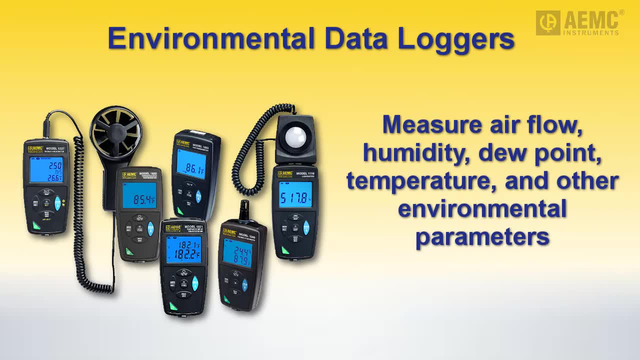 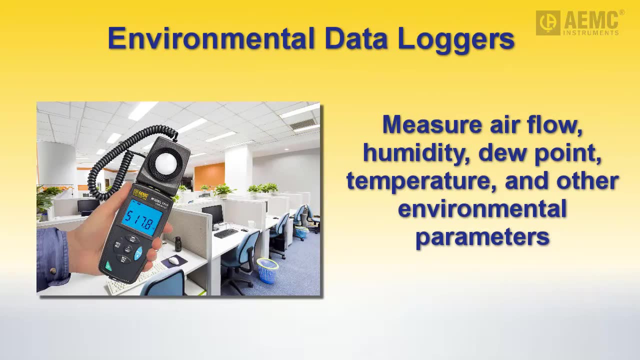 and perform other tasks directly on your Android smartphone or tablet. Other AEMC instruments can also help you monitor and improve the efficacy of your facility's heating and ventilation. For example, the AEMC Environmental series of data loggers record a variety of environmental quantities. 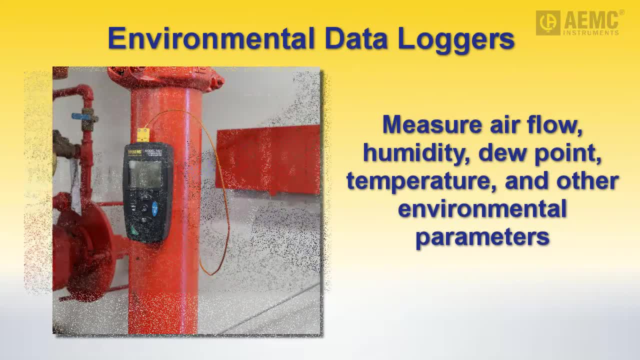 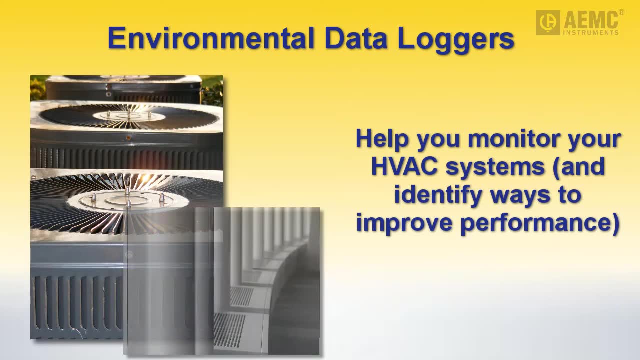 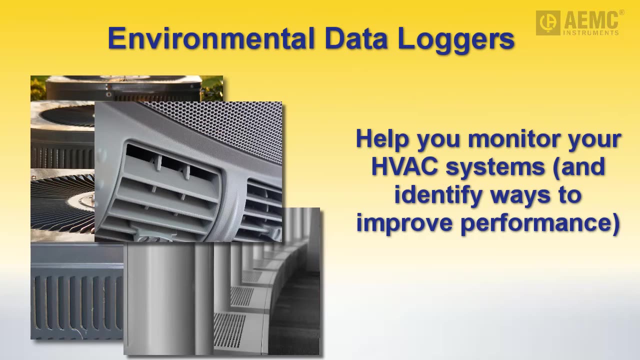 including air flow, humidity, dew point, temperature and other environmental factors. These instruments are especially useful for assessing whether or not your HVAC systems are performing efficiently and what types of fine-tuning may be required to ensure optimal performance. Let's take a moment to review. 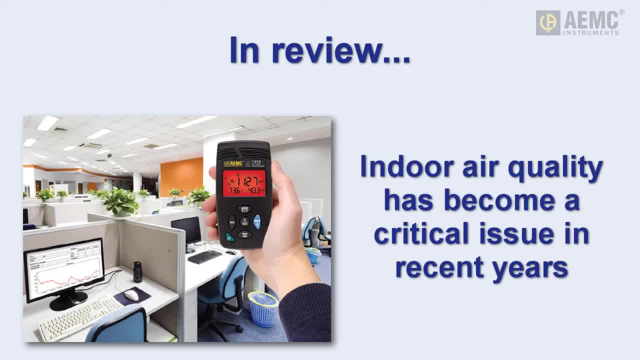 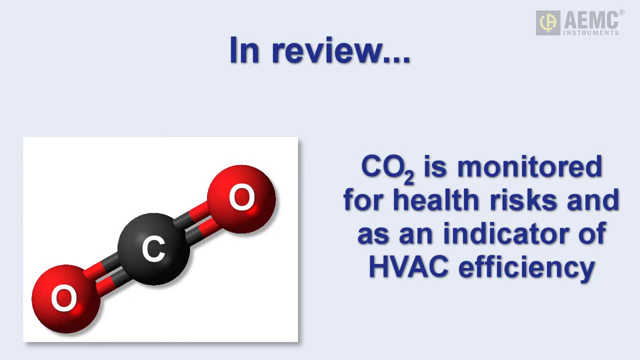 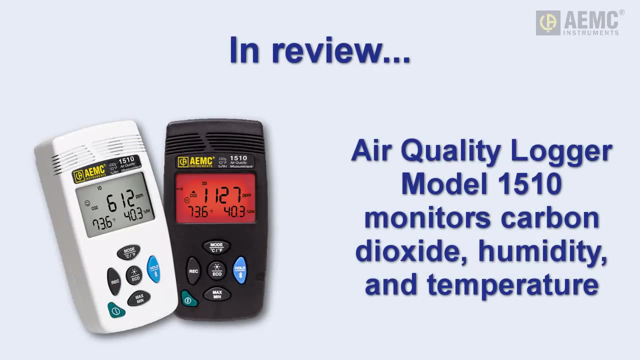 Indoor air quality has become an increasingly important issue in recent years. One particular area of focus is carbon dioxide, which can impact human health and performance, while also serving as an indicator of your ventilation system's efficiency. To help monitor the air quality in your facility, AEMC provides a variety of data loggers.